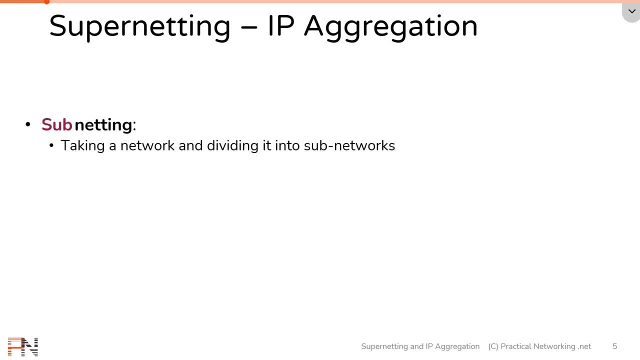 of Supernetting. In the Subnetting Mastery video series we define Subnetting as taking one network and dividing it into sub-networks. For example, if we started with 9.9.9.0.24,, that's a block. 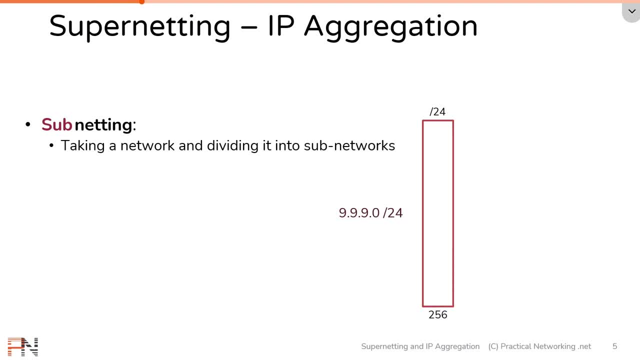 of 256 IP addresses. We can break that up into 2 slash 25s, each with 128 IP addresses, or 4 slash 26s, each with 64 IP addresses, Or 8 slash 27s, or 16 slash 28s, and so on. 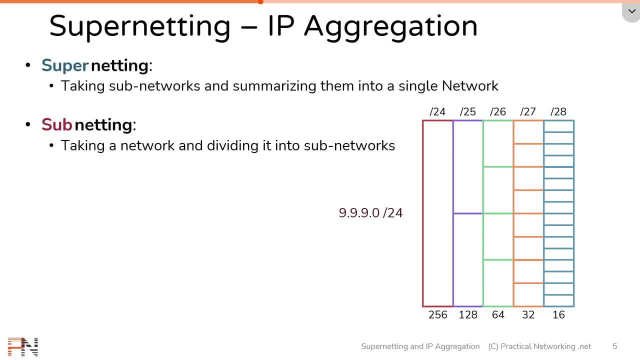 Supernetting is merely the opposite. It's taking those sub-networks and summarizing them back into single networks. I can take these 2 slash 28s and supernet them into that slash 27.. Or I can take these 4 slash 28s and supernet them into this slash 26.. 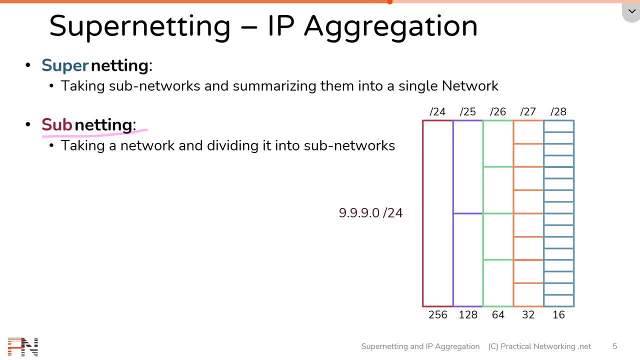 Understand that the terms Supernetting and Subnetting are relative to each other, Meaning this slash 26 is a supernet of these 4 slash 28s, But this 26 is also a subnet of this slash 25, or this slash 24.. So keep in mind, these terms are simply relative to 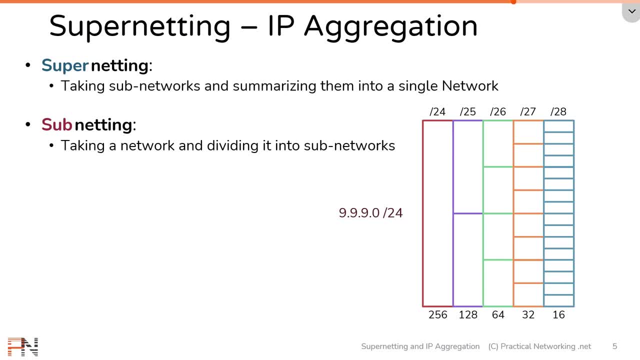 other networks or sub-networks. Also, I want to mention that the terms Supernetting, IP Aggregation and Summarizing are pretty much the same. They are interchangeable. They are simply different terms that all kind of mean the same thing. 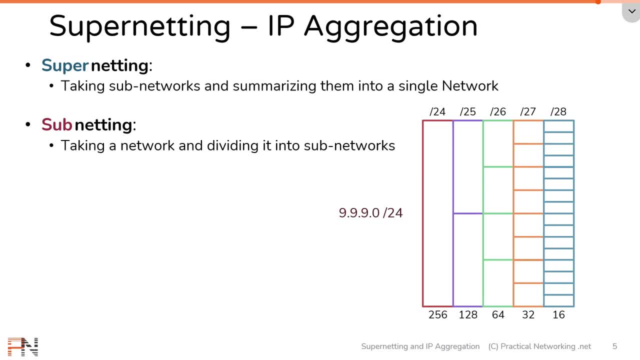 And with the definition out of the way, we are now going to show you how to use Supernetting. Let's get started. We are now going to show you 3 examples of Supernetting, each of which will show you different situations you will encounter when doing Supernetting. 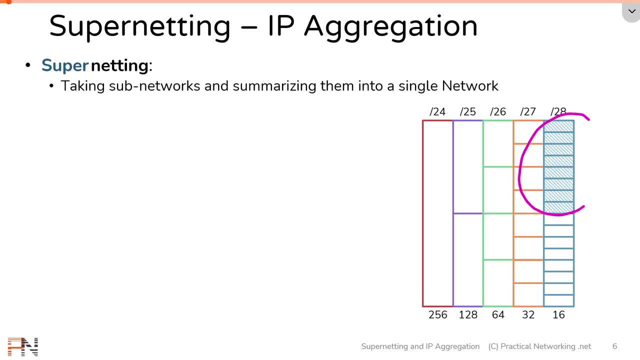 First, we are going to start by summarizing these 8 consecutive slash 28s. If you watched the Subnetting Mastery video series, then you are familiar with this chart. This chart tells us that slash 28 networks have increments of 16.. Which means the network. 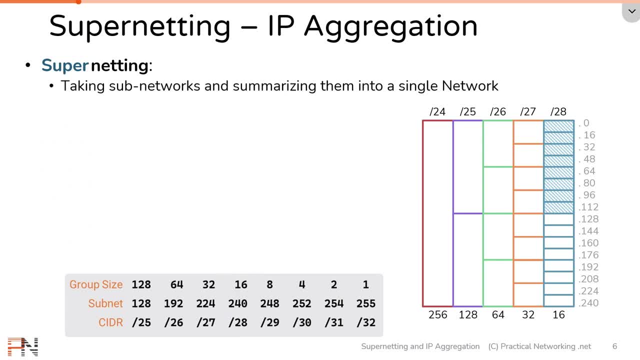 ID for all of the slash 28s we are trying to summarize. look like this: Now, if what we just did was a supernetting, then we are now going to show you 3 examples of Supernetting. If what we just did to figure out the increments and the network IDs was confusing, go ahead. 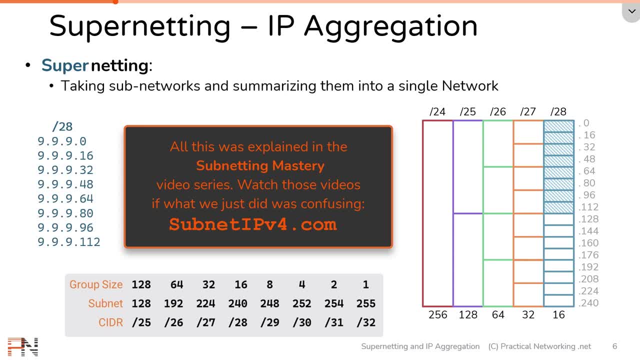 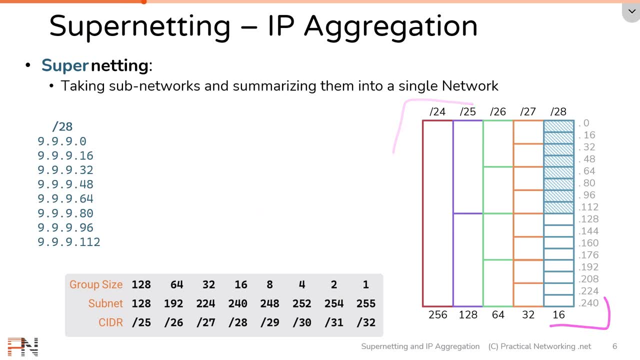 and pause this video and go and watch the Subnetting Mastery video series. This process is picked apart in great detail in that series. In any case, we are going to use this visualization to help us understand how to summarize these 8 slash 28s into fewer networks. 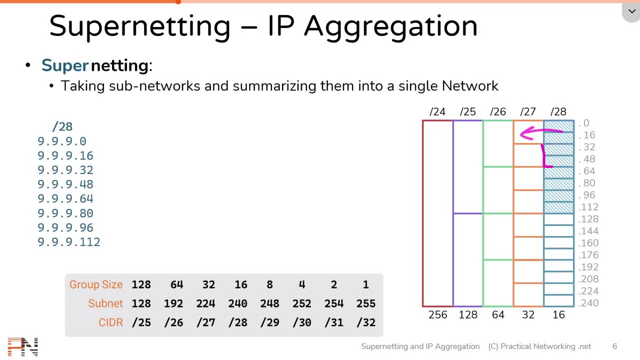 We can start by taking each slash 28 and summarizing them in pairs into their slash 27 counterparts. This would give us 4 equal slash 27s. 4 slash 27s are indeed aggregations of these 8 slash 28s, but we can go a step further. 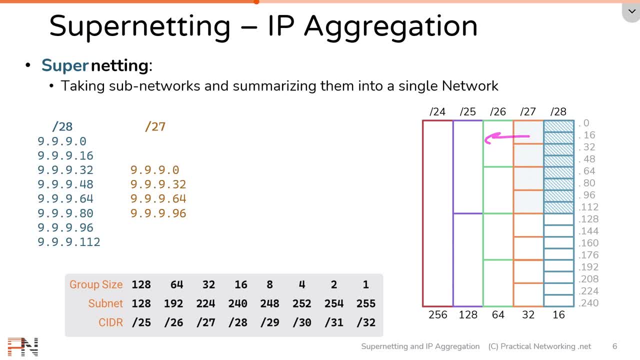 Notice: we can summarize these 2 slash 27s into a slash 26 and these 2 slash 27s into another slash 26, giving us a total of 2 slash 26s. These 2 slash 26s are the supernet of these 4 slash 27s and these 8 slash 28s. 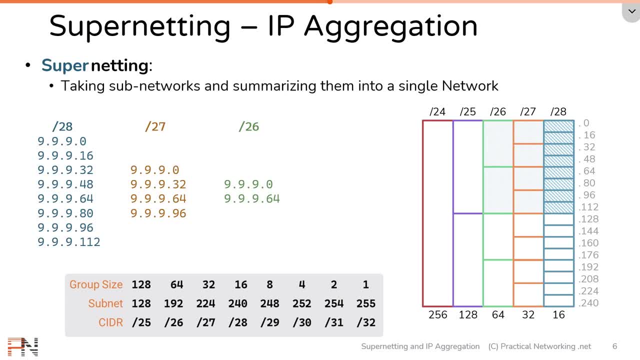 But can we do even better than that? Well, in this case, these 2 slash 26 are actually aggregates of the 8 slash 28s, and if we continue to use this visualization, we can see that these two slash 26s fit perfectly into. 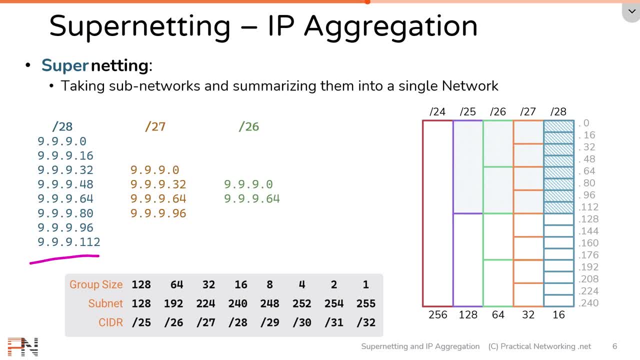 this slash 25.. Which means we can summarize these eight slash 28s or these four slash 27s or these two slash 26s into this one slash 25.. Now I do want to point out we could technically go further and summarize these into a slash 24.. Technically, the eight slash 28s we meant to 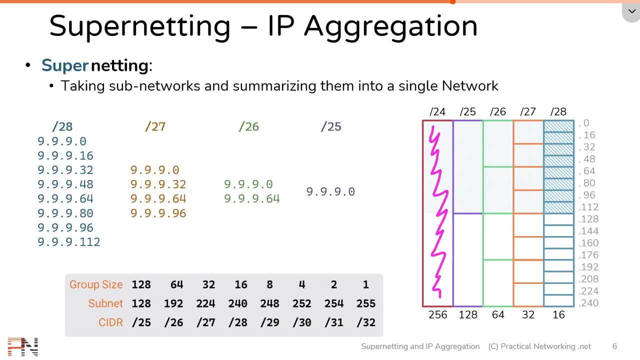 summarize absolutely fits inside this slash 24.. But if we summarize to the slash 24, we would be inadvertently also including IP addresses which we did not mean to initially include. In fact, we could even go a step further and summarize everything into 0.0.0.0.0.0.. That would include: 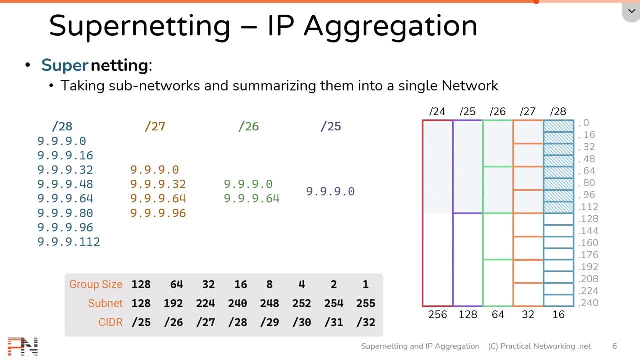 every IP address in the entire IPv4 internet, which certainly also includes these eight slash 28s that we are trying to summarize. But in both cases we could go a step further and summarize everything into a slash 24.. But in both of those cases, meaning the slash 24 or the slash 0, we were 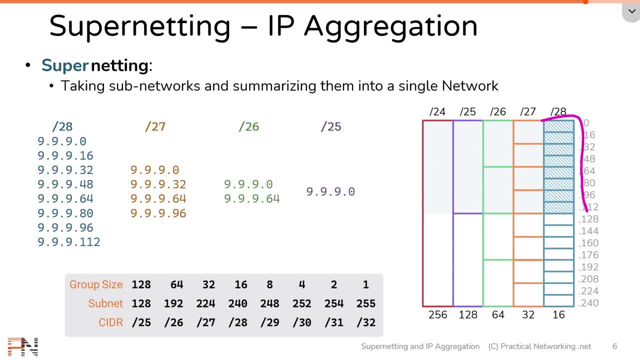 just discussing, we end up including more IP addresses than we mean. to summarize: Typically with supernetting you are trying to get to the smallest single network possible, which means 9.9.9.0 slash 25 is the best answer for this particular supernetting question. 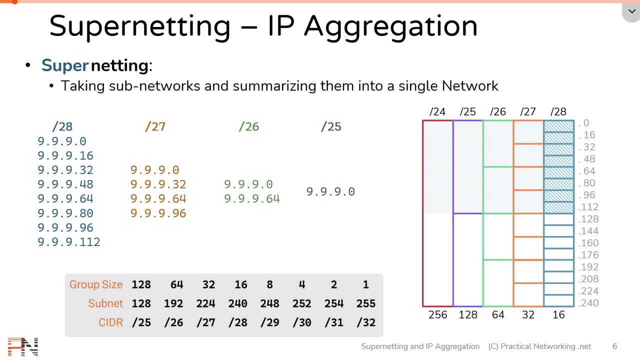 So we just went through our first simple supernetting exercise, But here's the thing: it isn't always going to work out as well as it did for this problem. Let me show you what I mean. Let's change our problem so that instead we are trying to summarize. 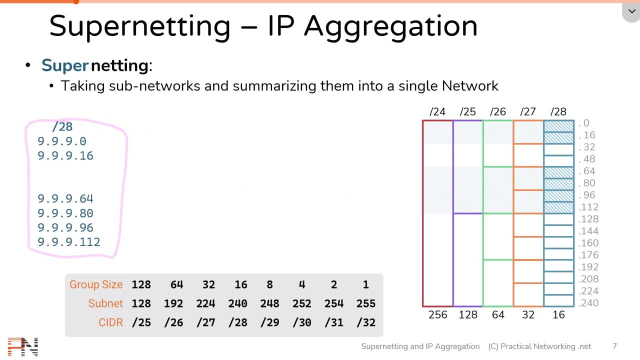 these six slash 28 networks. Notice we removed these two from our list. Well, these six networks are the ones that we are trying to summarize, So we are going to do this in the same way that we did in the previous example, But notice that the six slash 28s still. 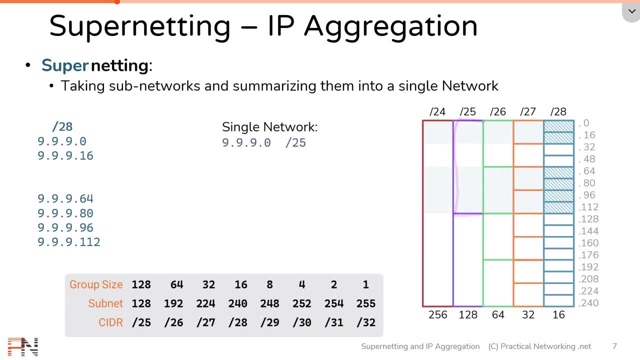 fall in the exact same slash 25.. So if we wanted to summarize these into a single network, we could still do so with 9.9.9.0, slash 25.. But notice, this slash 25 is now including IP addresses which we did not mean to summarize. And if you look at this visualization, 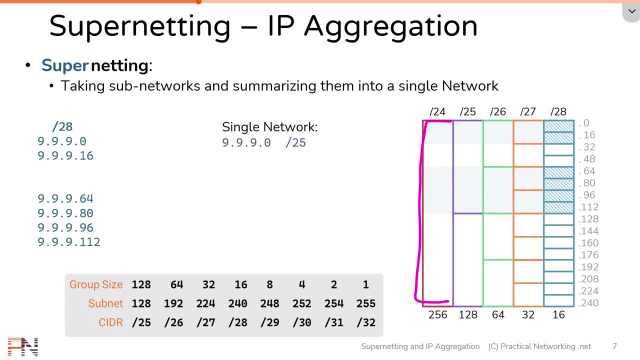 we can see that there really isn't a way to go a step bigger or a step smaller without also including IP addresses. we didn't mean to summarize or excluding IP addresses, we did mean to summarize. So you see, sometimes when you are doing, 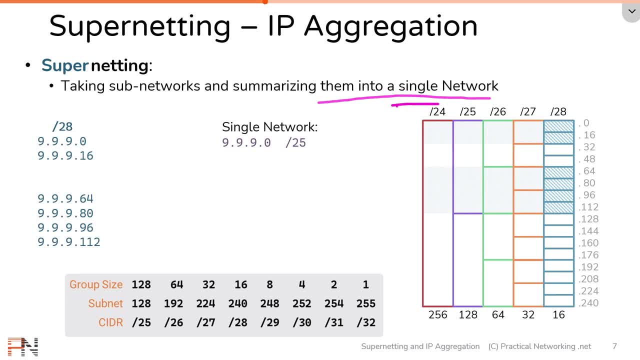 supernetting. your target is to summarize everything into a single network, But other times your target is going to be to summarize into as few networks as possible. In this case, if we wanted to match these six slash 28s exactly, we would have to summarize. 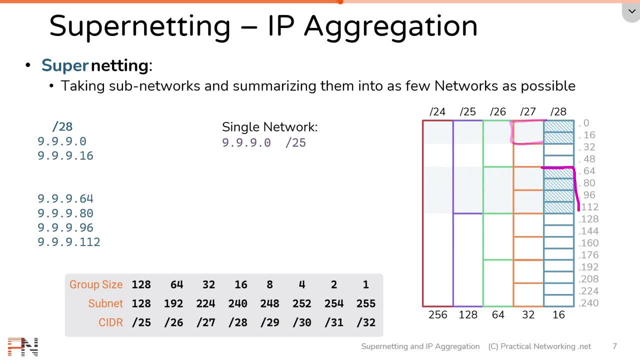 these two slash 28s into this slash 27,, and these four slash 28s into this slash 26,, giving us an exact match result of these two networks. Okay, so which of these is the correct answer then? Well, both. It depends on what the question is asking, or what it is that you're trying to. 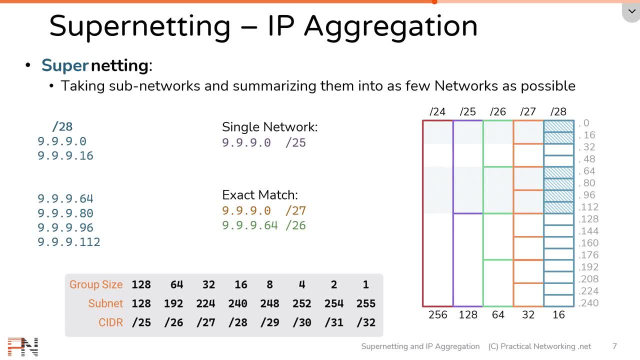 accomplish. If you're trying to do something like routing, where you're trying to direct traffic for these set of IP addresses to a particular next hop, then it might be safe enough to simply use a single route with a slash 25.. But if you're doing something like 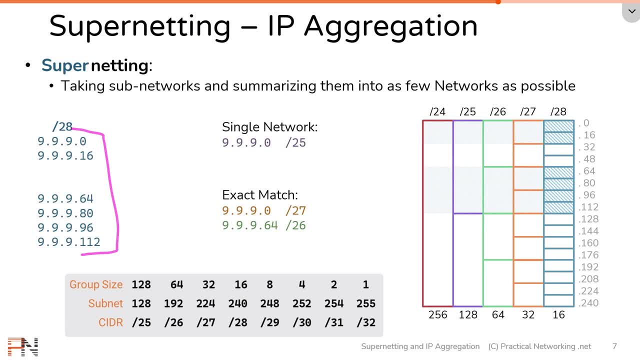 routing between the dashed network and the access control list, which involves giving access from these IP addresses to specific resources, then maybe you want to be more explicit with who you're trying to give access to and would therefore want to use an exact match. 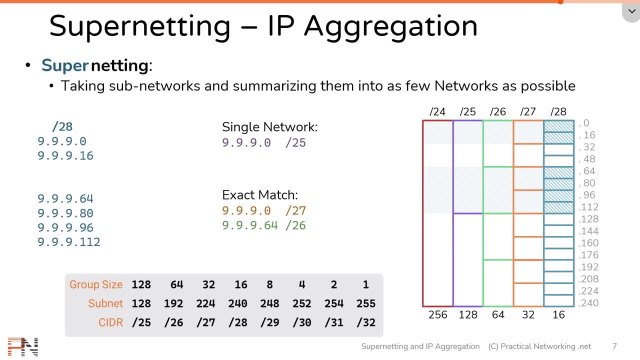 So both of these can be right answers And when faced with supernetting problems, you'll have to infer from the question text or the task at hand whether it makes more sense to supernet to a single network and potentially include IPs you didn't mean to, or supernet to as 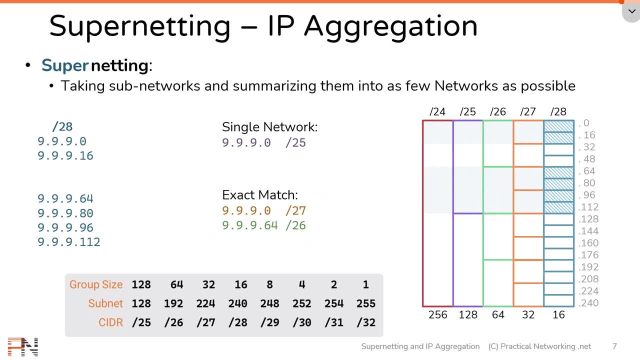 few networks as possible, multiple lines in your configuration. so that's the idea behind summarizing to a single network or an exact match. now there's one more example I want to show you. let's do one more of these together before I test you, to see what you've. 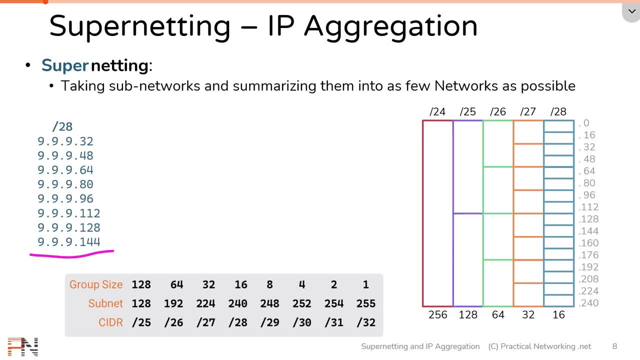 learned. let's now try to summarize these eight consecutive slash 28. each of these slash 28 has 16 IP addresses and if you do 8 times 16, that does indeed get you 128. and if we look at this chart, we can see that a slash 25 network has exactly. 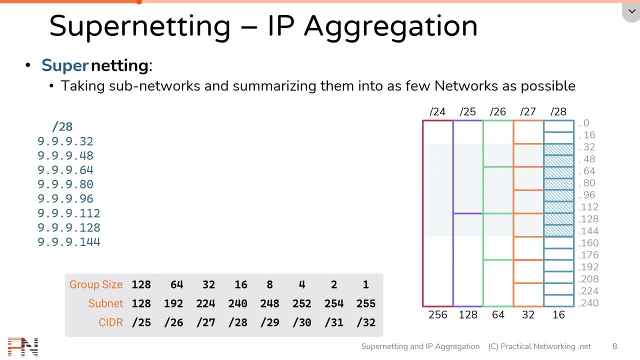 128 IP addresses, which means a slash 25 has enough IP addresses to hold these eight slash 28. this is how we were able to summarize the 8 slash 28 from our first problem into a single slash 25. but take a look at where these 8 slash 28. 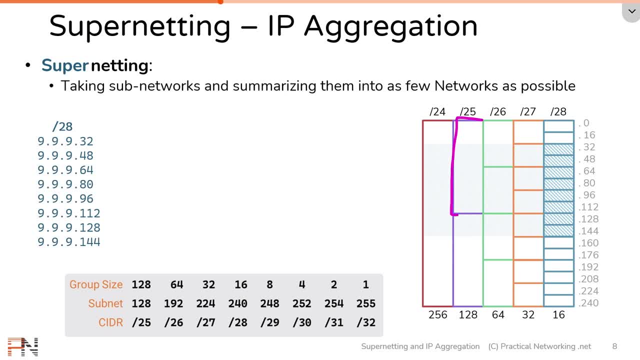 fall. if I try and summarize them as 9.9.9.0 slash 25, I would only be accounting for the these top six slash 28s, and if I try and summarize them as 9.9.9.128 slash 25, I. 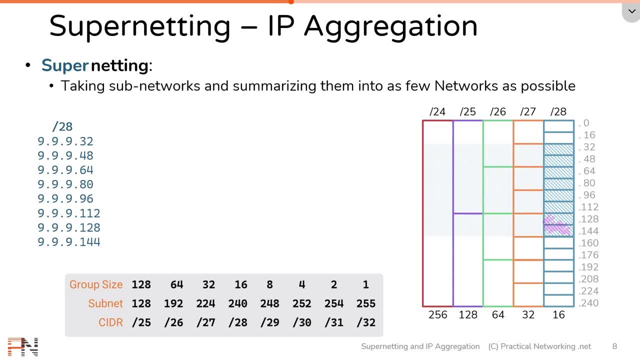 would only be accounting for these two slash 28s. you see, slash 25s always fall either on dot 0 through 127 or on dot 128 through dot 255, even though a slash 25 has enough IP addresses to account for all the slash 28s. we need to summarize. 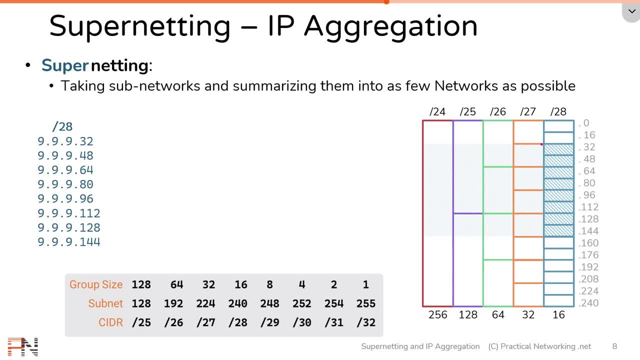 there is no slash 25 that starts on dot 32 and ends on dot 159.. so for this particular prom, because of where the subnets are that we are trying to summarize, we actually have to go a step further and summarize all of these into a slash 24.. that's the only option. 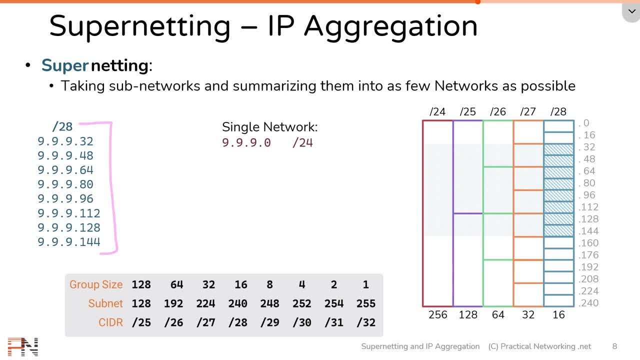 we have to summarize all eight of these slash 28s into a single network. of course, summarizing to the slash 24 also makes us include a bunch of IP address space that we didn't mean to include as a common side effect when you're trying to summarize to a single network. 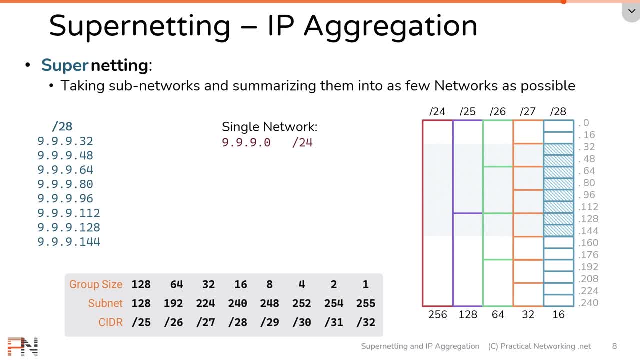 instead, if you want to summarize for an exact match, we could summarize these two slash 28s into this 27, these four slash 28s into this 26 and these two slash 28s into this 27, giving us an exact match summary of these three networks. at this point, we've worked through three summarization. 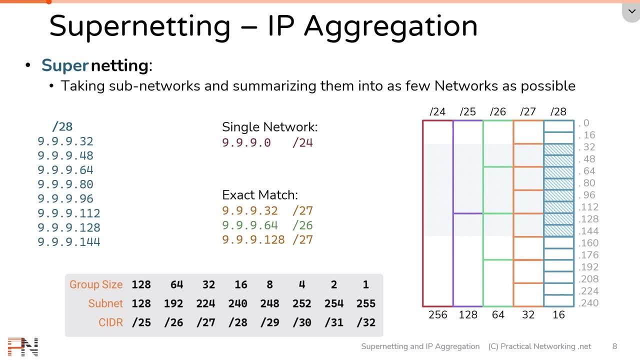 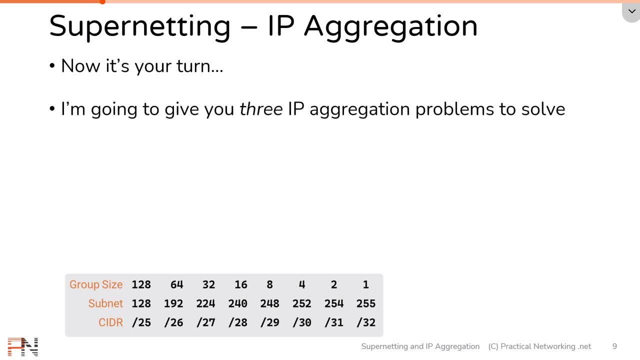 problems together. both of these progressively showed you some of the nuance that is involved when doing IP aggregation. now it's your turn. I'm going to give you three IP aggregation problems, just like we just did for you to solve. for each of them, I want you to solve two things. I want you to summarize every. 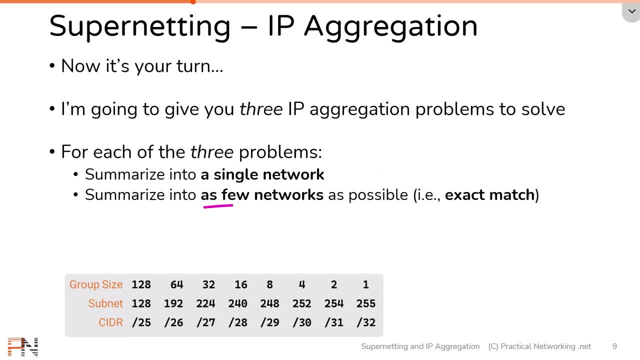 network into a single network and I want you to summarize every network into as few networks as possible, meaning summarized to exact match. these three problems happen to be on the next slide and I'll mention that on the slide I don't have room for this subnetting chart, so you might want to quickly grab a. 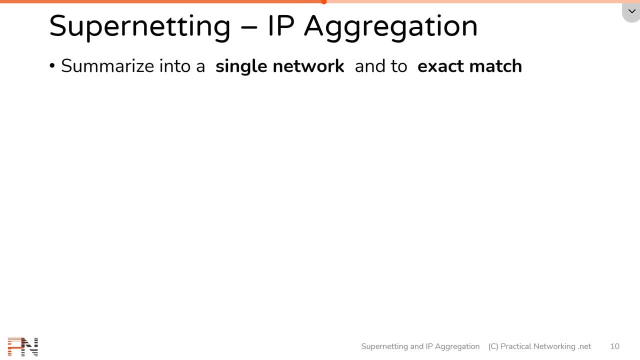 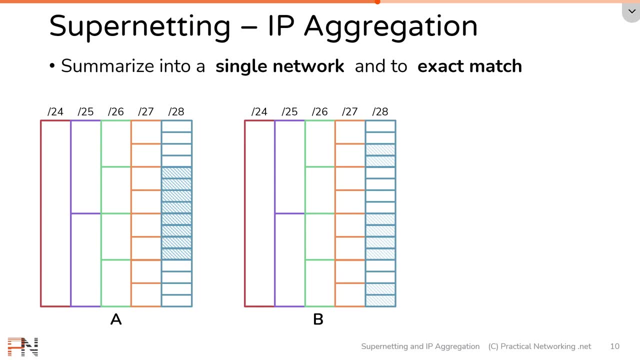 screenshot or jot this down. Either way. here are your three problems. Problem A is going to have you summarize these eight consecutive slash 28s. Problem B is going to have you summarize these eight non-consecutive slash 28s. And finally, problem C will have you summarize a mixed set. 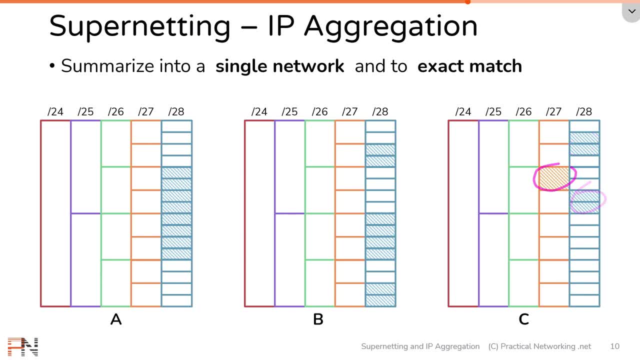 of networks, some slash 28s and a slash 27.. So go ahead and work through these aggregation problems and again, for each of these, solve for two things: summarize everything to a single network or to an exact match. Go ahead and pause this video to work on these problems. I'll reveal the answers in 10. 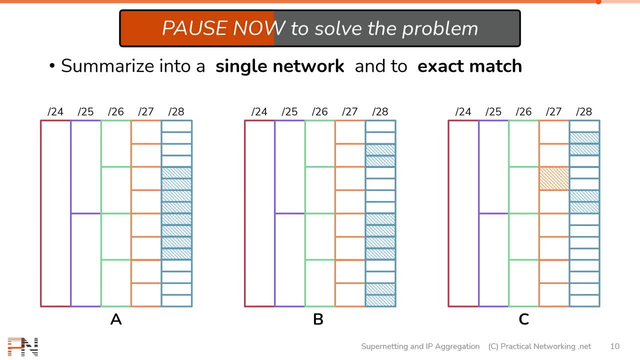 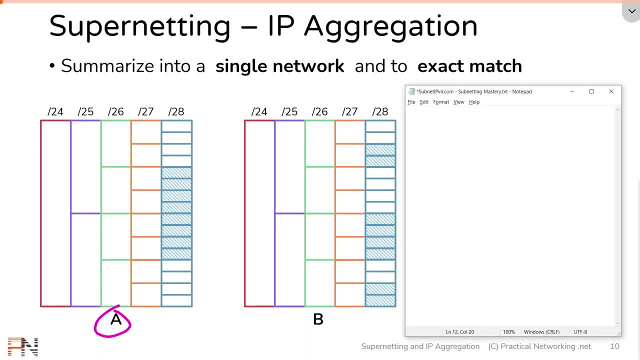 seconds For problem A. to summarize these eight slash 28s to a single network, the only option you have is to summarize to the entire 9.9.9.0. slash 24. And to summarize them to an exact match. you can take these four and summarize them to this. 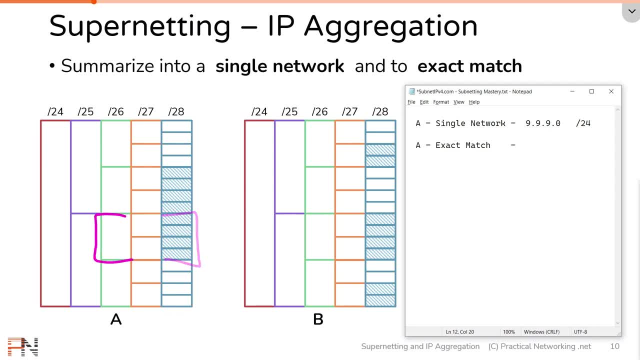 slash 26 and these four slash 28s and summarize them into that slash 26,, giving us an exact match value of 9.9.64 slash 26 and 9.9.128 slash 26.. For problem B, to summarize to a single network, 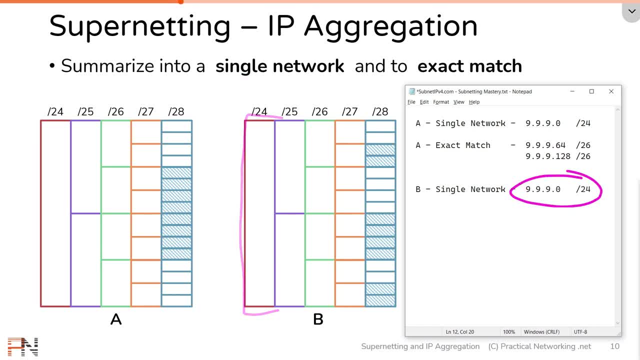 again, your only option is to summarize everything to 9.9.9.0 slash 24.. And to summarize to an exact match, you can take these two slash 28s and summarize them into a slash 27,. these four slash 28s and summarize them into a slash 26.. And finally, these two slash 28s and summarize them. 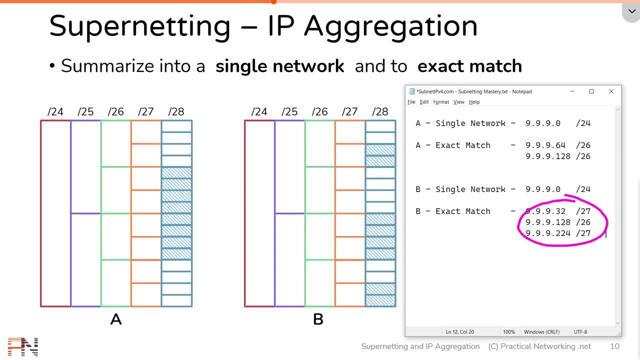 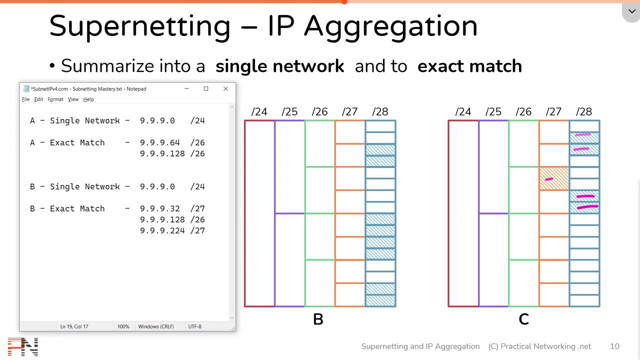 into this, slash 27,, giving you an exact match value of 9.9.9.32 slash 27,, 9.9.9.128 slash 26 and 9.9.9.224 slash 27.. And finally, for problem C, to summarize all five of these networks into a. 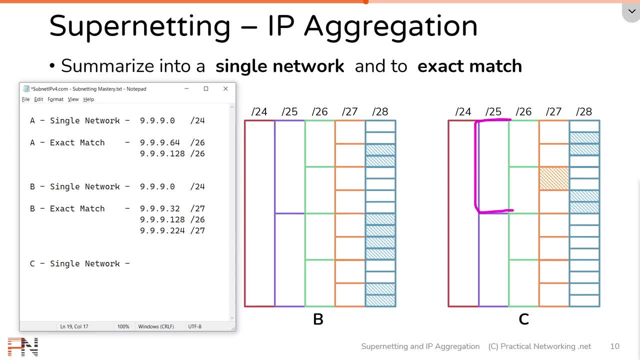 single network. you can use this slash 25, giving us a single network answer of 9.9.9.0- slash 25.. And summarizing them to an exact match you're going to see is going to be a little tricky. 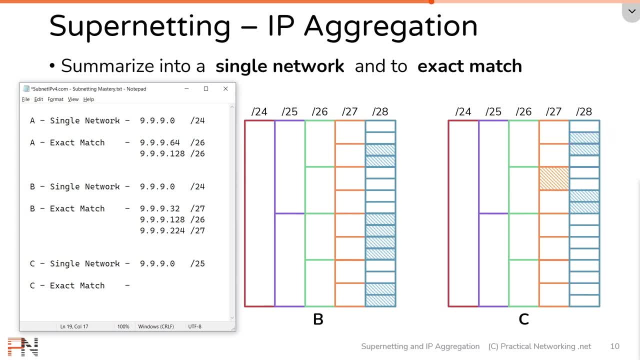 This slash 28 actually cannot be summarized into anything else. The next size network would be a slash 27, and it includes IP space. we didn't mean to summarize, So this slash 28 has to stay as a slash 28.. And it's the same for that slash 28 right there. Because of where these 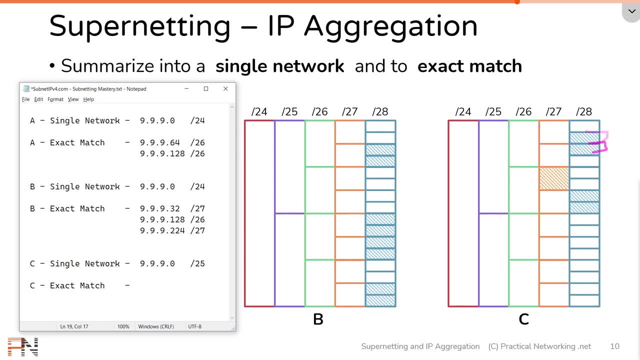 27s fall, there is no way to summarize those two slash 28s. This slash 27 and these two slash 28s can both be summarized into this slash 26,, giving us an exact match. summarization answer of these three networks. Notice, the two slash 28s are the two original slash 28s we meant to summarize. 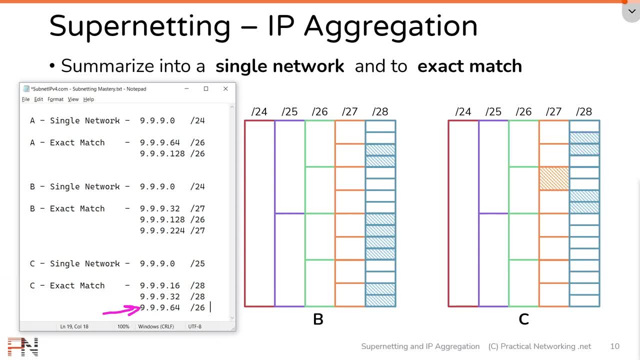 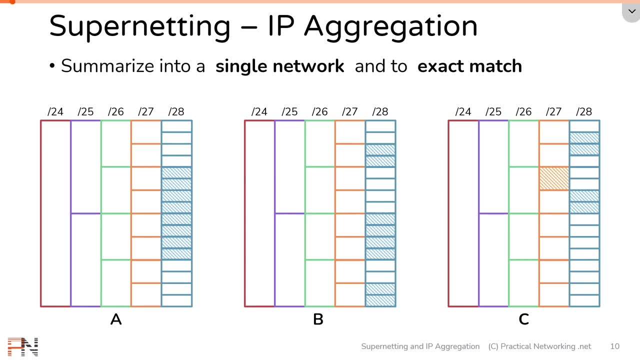 The only one we were actually able to summarize was this guy down here summarizing these networks into this slash 26.. So at this point you've seen six supernetting problems. We did three together in the beginning and then just now we tested you on these three problems. Hopefully now you 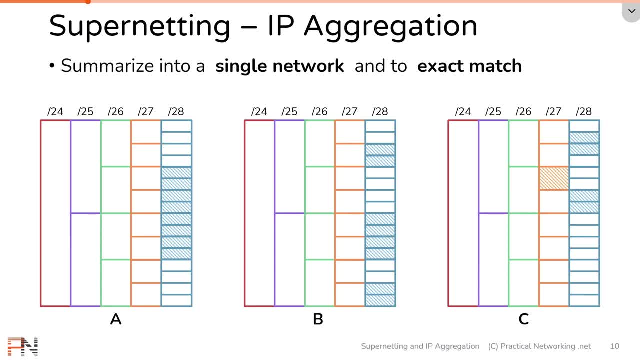 understand what supernetting problems are asking you to do And hopefully you've come to realize that it isn't a very difficult task- Or at least it isn't difficult if you have these cool visualizations of all the IP addresses and different subnet blocks. that'll help you find. 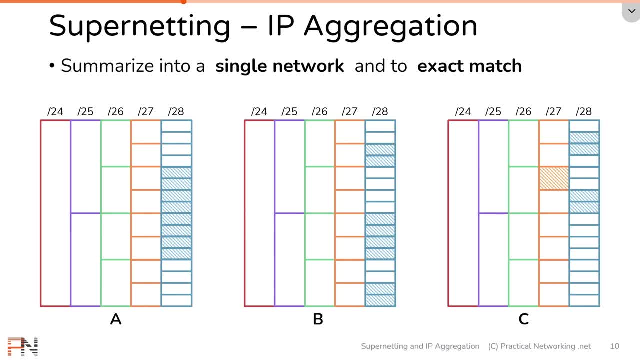 the right answer. But in the real world or on a certification exam, you aren't really going to have the luxury of this cool table. But, lucky for you, you can solve supernetting problems using only scratch paper, and that is what I'm going to show you next. Now, I do want to mention that 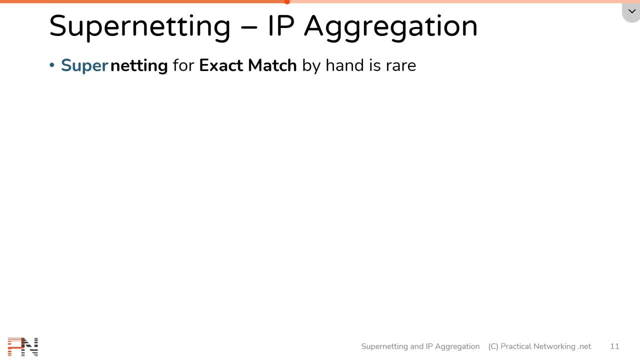 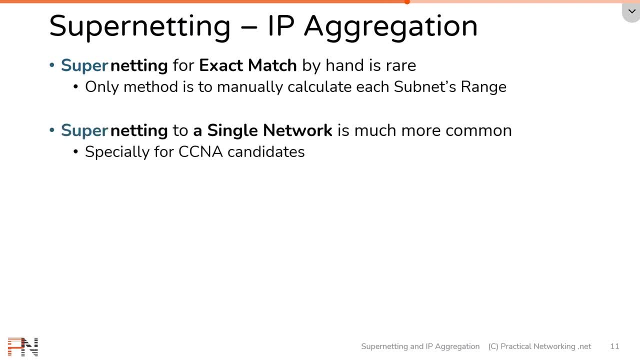 Instead, much more commonly, you'll be asked to supernet, to a single network. You'll be given certain subnets or certain IP addresses and you'll be asked to find a single network which they all fall into. Luckily, this is something that is pretty easy to do quickly, and I'm going 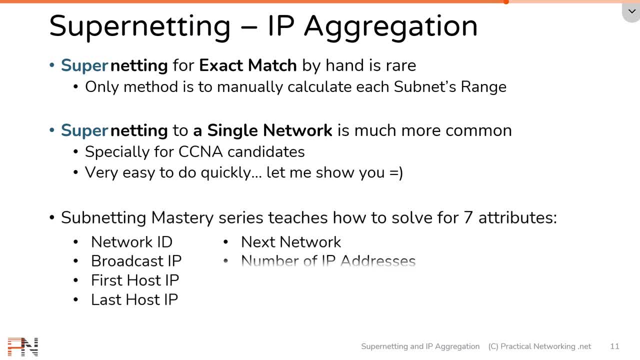 to show you how, In the subnetting mastery video series, I taught you how to solve for these seven attributes. I told you that every subnetting problem you ever encounter is simply asking you to solve for one or more of these values. Well, for supernetting you're going to need: 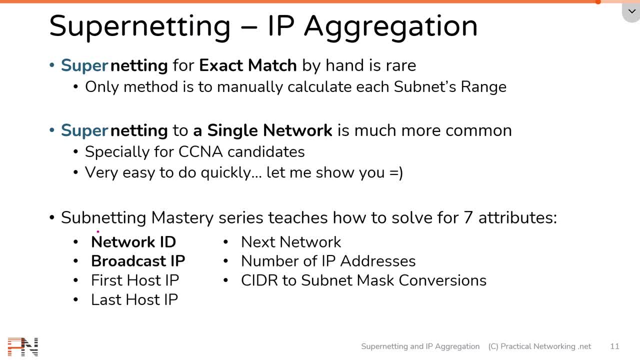 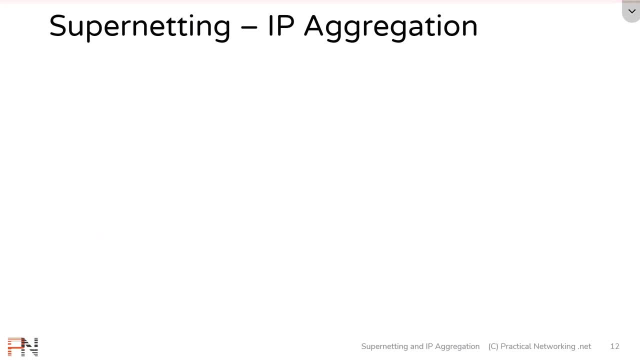 one or more of these values For supernetting. the two attributes we'll be using are the network ID and the broadcast IP. So let me show you how to use these two values to solve supernetting problems. We're going to start by summarizing these six, slash 28s If these 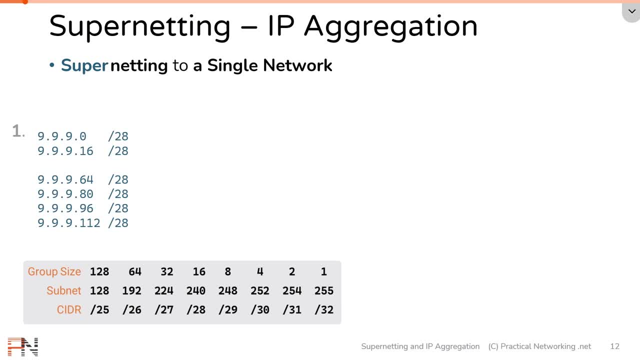 look familiar to you, it's because it's the same slash 28s we worked through earlier. I just wanted to start with something familiar. Supernetting by hand only requires two steps. The first step is to find the smallest IP address and the largest IP address. Now notice: I said IP address and not subnets, So the 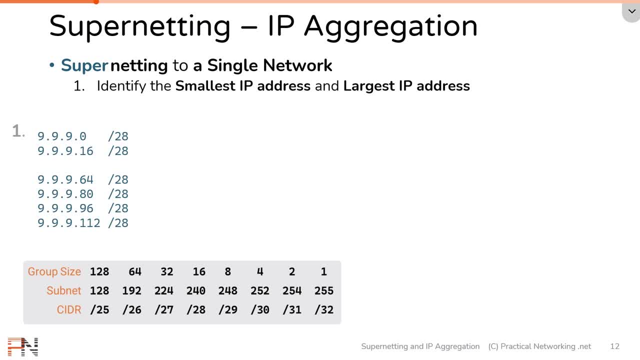 smallest IP address. for our problem set is going to be the network ID of the lowest numerical subnet, meaning this one. And since this problem has already given us the network ID, we know that the smallest IP address is going to be 9.9.9.0.. Then we're going to try and find. 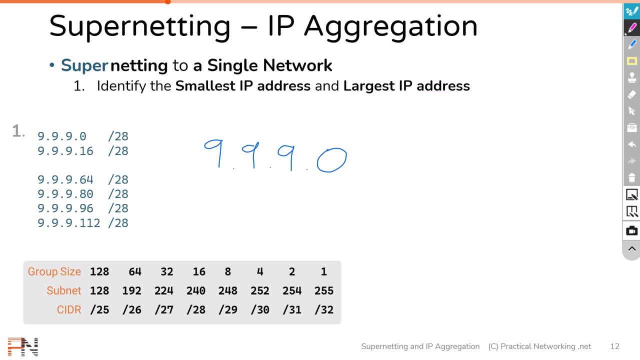 the largest IP address. The largest IP address is going to be the last IP address in the highest numerical subnet, which is going to be that one. Now, the last IP address in that subnet is the broadcast IP address. So we simply have to solve for the broadcast IP of this subnet. Well, this: 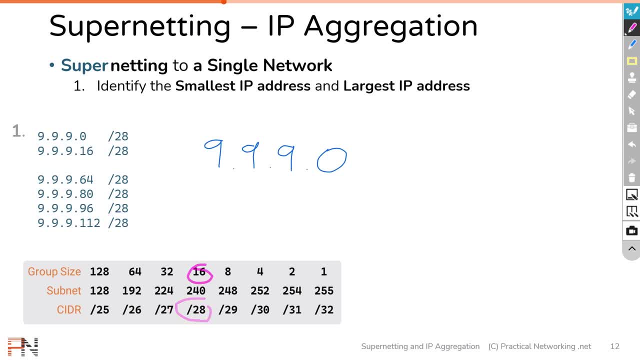 is a slash 28,, and a slash 28 has an increment of 16.. So if we add 16 to 112, we would get 128.. Of course, 128 is the next network value, so we have to do minus 1 to get us a broadcast. 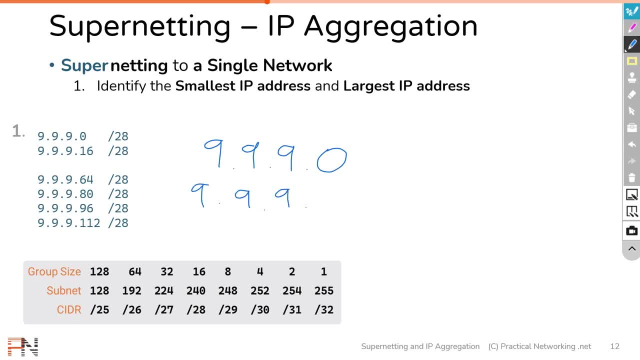 IP address. So we're going to have to add a new network IP address of 9.9.9.127.. Now, everything we just did insofar as solving for the network ID and broadcast is stuff we covered in the Subnetting Mastery video series. So if you're unsure how I solved, 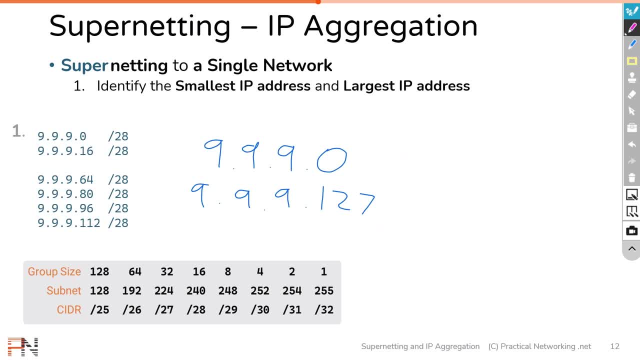 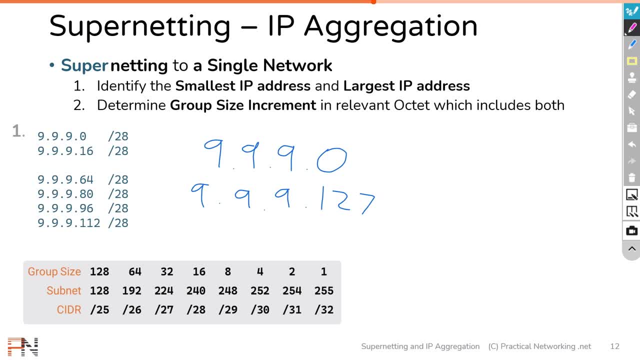 That includes both the smallest and largest IP address. So if we subtract 127 from 0, we get 127. So we know that we need an increment that is at least 127.. This means all of these are too small, all the way until I get to a slash 25.. A slash 25 has an increment of 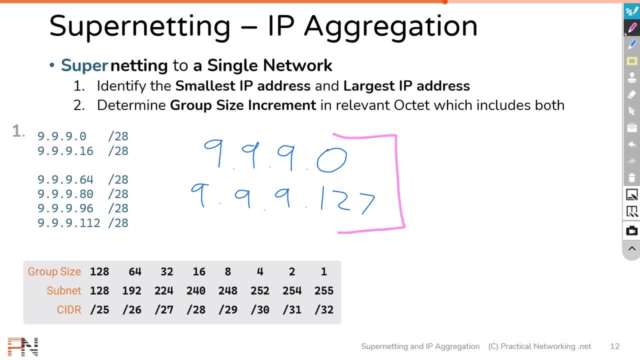 128,, which is enough to account for the jump we need, And since there's a slash 25 that starts at 9.9.9.0,, this gives us our answer. The supernet of these 6-slash-28s is 9.9.9.0-slash-25.. 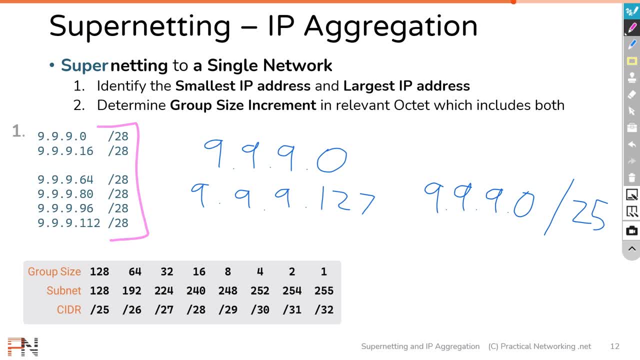 Just like that we were able to solve for the supernet of these 6-slash-28s. You'll notice we got the same answer as we did when we used the large chart and did this visually. Notice we didn't have to do anything with the IPs and subnets in the middle. 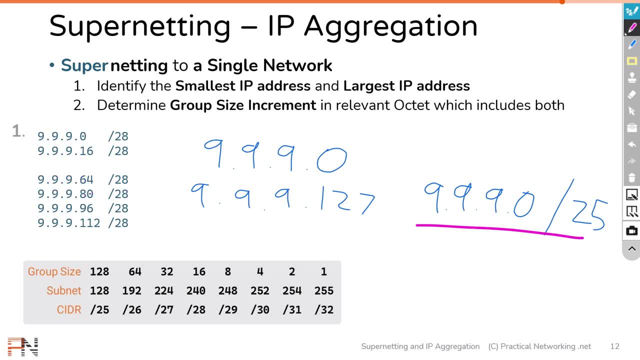 The thing is, if we find a subnet that includes the smallest IP address and the largest IP address, it's definitely also going to include all the IP address space in the middle, And just like that, with only these two steps, we have solved our first supernetting problem. 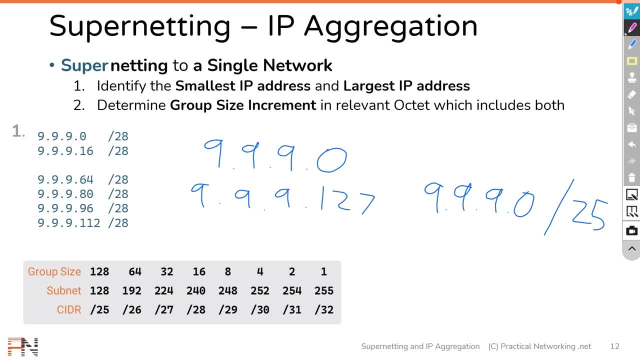 But I want to show you a few more examples. I have five more problems that we are going to work through together and, as before, each of them will show you something different. in regards to supernetting, For the next problem, we're going to use the same problem as the first problem. 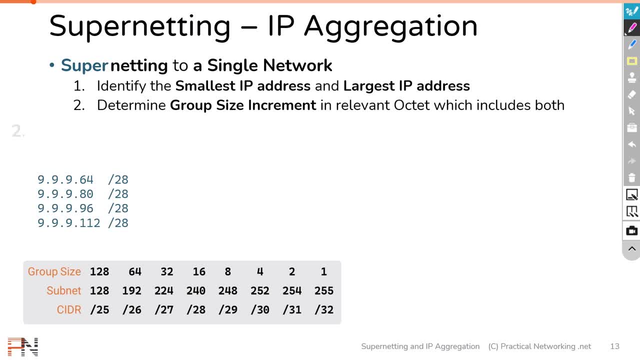 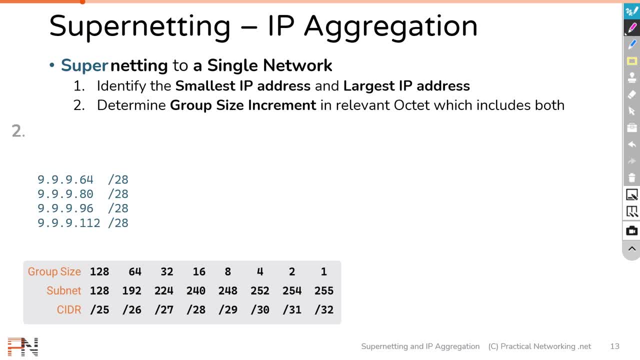 And we're still going to use the exact same two-step process. First we'll start by identifying the smallest IP and the largest IP, And the smallest IP address will be the network ID of that subnet, right there. So our smallest IP address is going to be 9.9.9.64.. 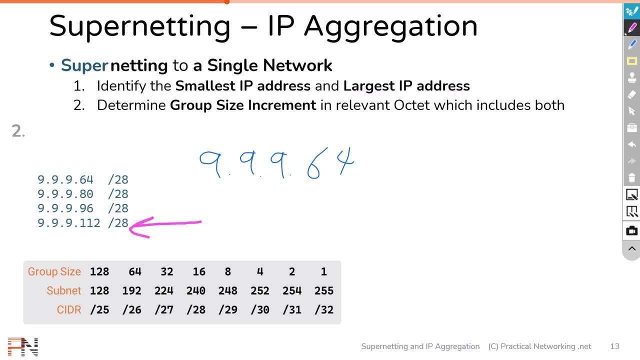 The largest IP address is going to be the broadcast IP address of the highest numerical subnet. The broadcast IP address will be the subnet, which for us is 9.9.9.112 slash 28.. Now, this is the same subnet as last time, so the broadcast IP address hasn't changed. 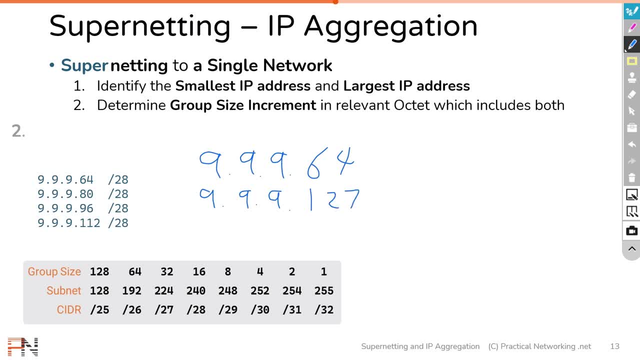 We know that it's 9.9.9.127.. And from here we'll just find an increment that includes both the smallest and largest IP address. Well, if we do 127 minus 64,, that gets us 63,, which means all of these are too small. 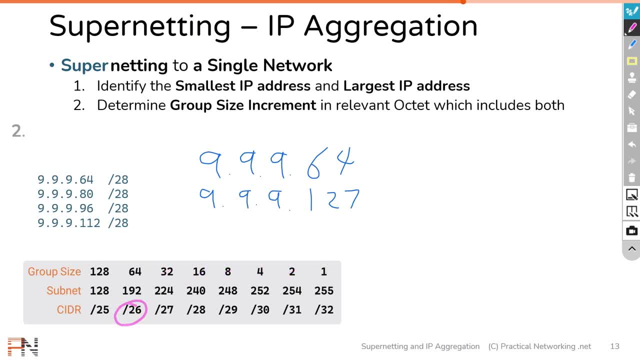 until we get to 64, which is a slash 26.. And since a slash 26 happens to start on 9.9.9.64,, right away we have our answer of 9.9.9.64, slash 26.. 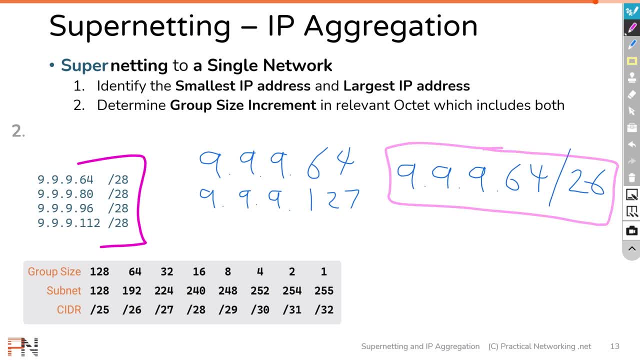 This right here is the supernet for these four slash 28s, And just like that we have solved another one using these two steps. Let's do one more. Our next problem is going to involve supernetting mixed-size networks. Notice, here we have a slash 29,, a slash 27,, a slash 26, and a slash 28.. 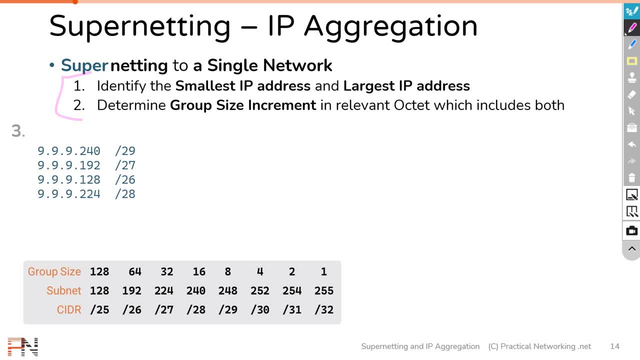 We're going to still use the same two-step process to find the supernet. We'll start by identifying the smallest IP address, which is going to be the network ID of the lowest numerical subnet, which, for us, is going to be that guy right there. 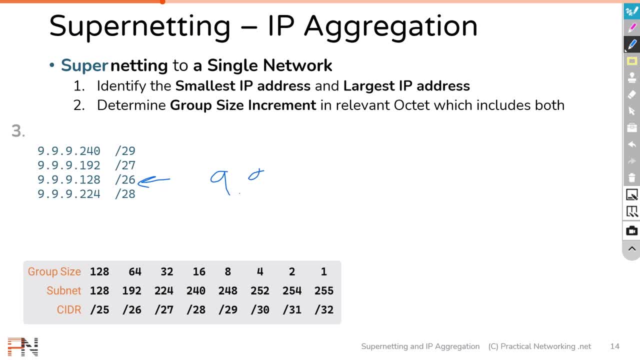 which means our smallest IP address is going to be 9.. 9.9.9.128.. Our largest IP address is going to be the broadcast IP of the highest numerical subnet, which for us looks like this guy right there: This is a slash 29,, which is an increment of 8,. 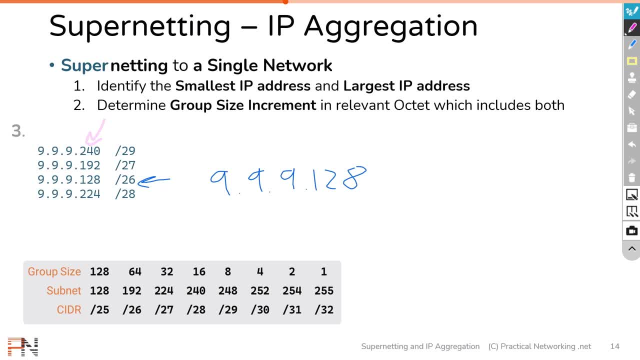 which means if we add 8 to that guy, we get 240. plus 8 gets us 248.. Again, that's the next network. So if we do minus 1, that'll give us the broadcast IP of our largest numerical subnet. 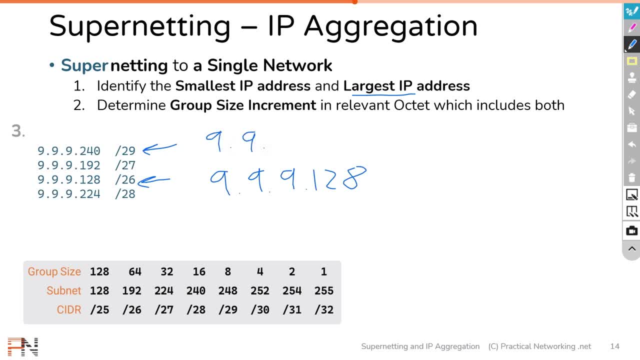 which means our largest IP address is 9.9.9.247.. And again, we now just need to find a group size increment which includes both the smallest and largest IP address. If we do 247 minus 128,, that gets us 119,. 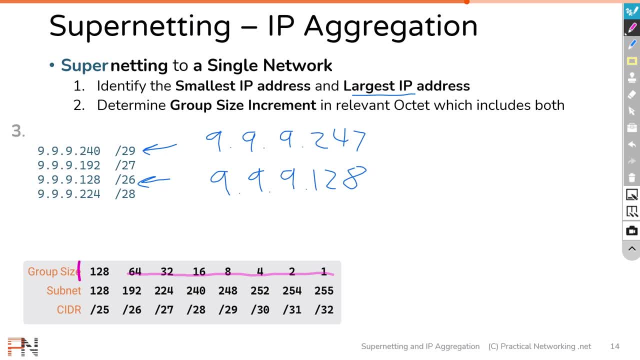 which means instantly, we can rule out all of these networks and go straight to a slash 25,, which is the first network that is big enough to account for this jump. And since there happens to be a slash 25,, we can go straight to a slash 25,, which is the first network that is big enough to account for this jump. And since there happens to be a slash 25,, 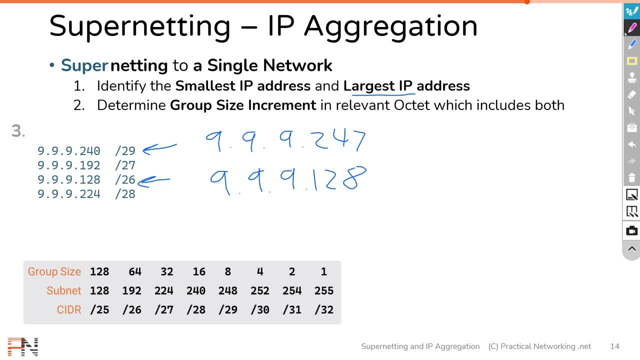 And since there happens to be a slash 25, that starts on our smallest IP address, .128,, we instantly know that the answer to this supernetting problem is 9.9.9.128, slash 25.. So that is our third supernetting problem. 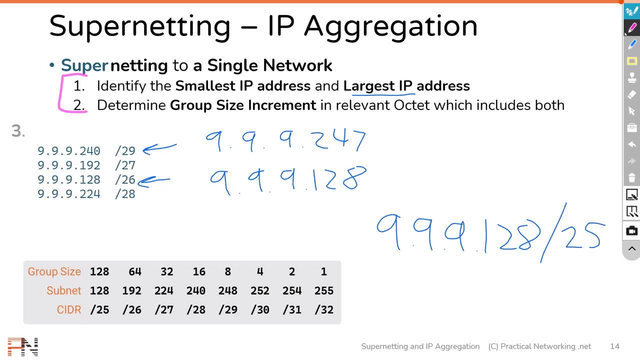 And again you'll see we just used those two steps And this time we summarize networks of mixed sizes. So far, every supernetting problem we've worked through together has been using subnets, But occasionally you're going to run into supernetting problems that involve summarizing individual IP addresses. 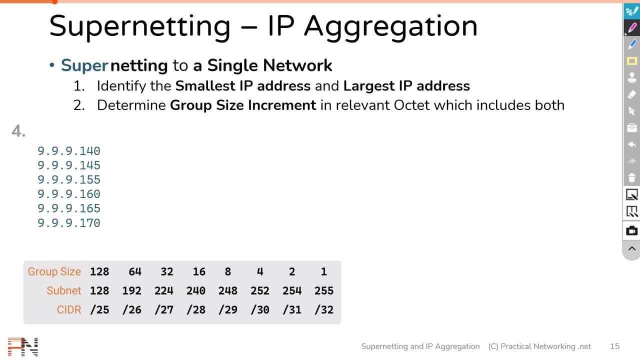 Well, either way, the same two-step process will work to solve the supernet. Again, we're going to start by identifying the smallest IP address, which for us looks like this guy, and the largest IP address, which for us looks like this guy. 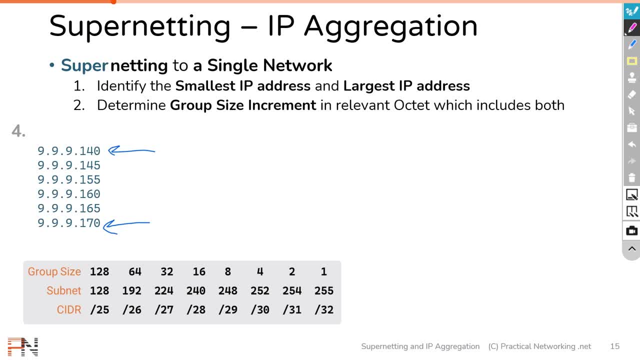 Since they've already given us IP addresses, we don't need to calculate network IDs or broadcast IPs. We can go straight to step two, which is to find a group of IP addresses, a group size increments that includes .140 and .170.. 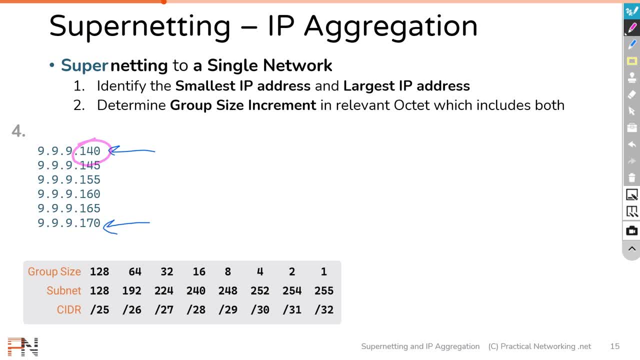 Now, if you subtract 170 from 140, we get 30, which means we need a jump of at least 30. This lets us rule out all of these networks until we get to a slash 27.. But we have to be careful here. 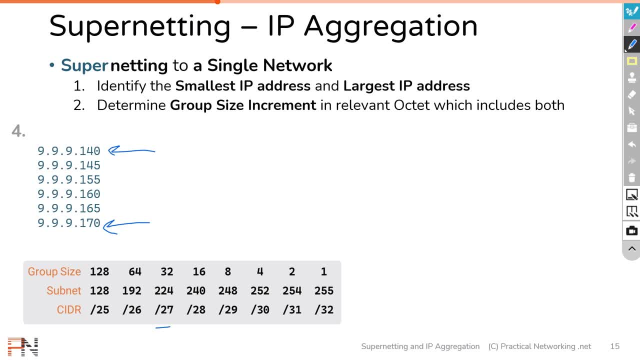 If we take slash 27 networks and we list out their increments in sets of 32, you would get .0, .32, .64.. Now, of course, in the subnetting mastery video series, I showed you some speed tips that'll let you speed this process along. 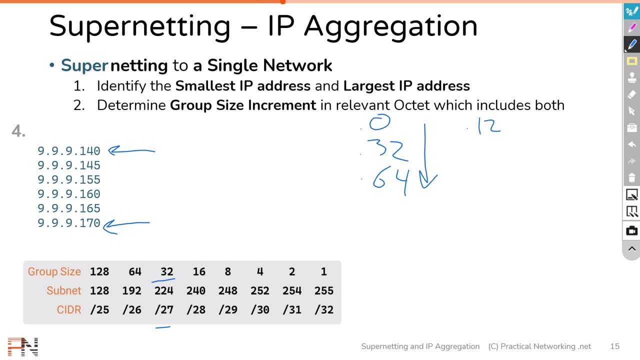 One of those speed tips told us we can simply start from 128.. Again, if you haven't seen that series, definitely check that out. I go into more detail about these shortcuts Either way from 128, if we continue in sets of 32,. 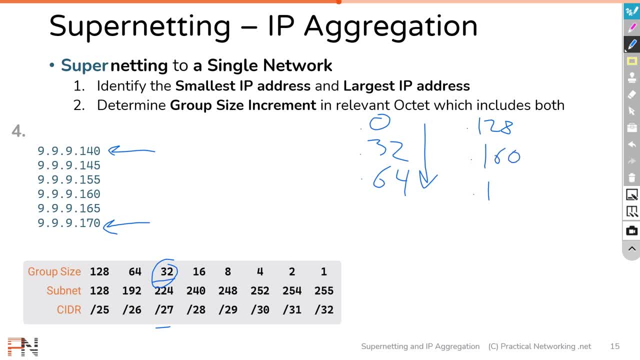 we would get 160,, then 192, and we can stop here. Notice the IP addresses we are trying to solve: 140 through 170, start somewhere in here and end somewhere in here in the next block, which means, even though a slash 27 is enough IP addresses to account for this jump. 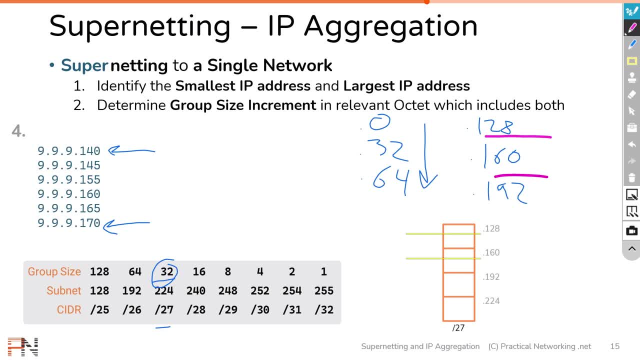 these two addresses happen to exist in two different slash 27s, which means a slash 27 is not going to be big enough to include this entire set. Instead, we have to go one step further and go to a slash 26.. The increment of slash 26 is 64.. 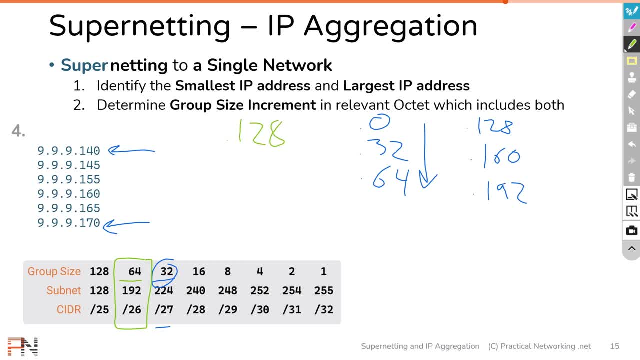 And if we start at 128, the next increment is going to be 192.. And between these two values we do have enough to include all the IP addresses. we're trying to summarize, which means the answer to this supernetting problem is going to be 9.9.9.128.26. 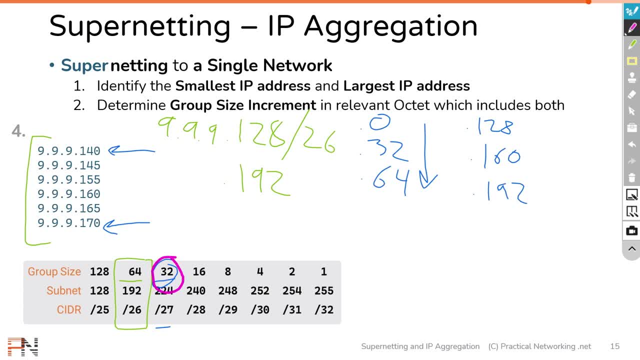 So keep in mind: just because you have enough IP addresses doesn't necessarily mean you're going to be able to solve all the IP addresses. So keep in mind: just because you have enough IP addresses doesn't necessarily mean you're going to be able to solve all the IP addresses. 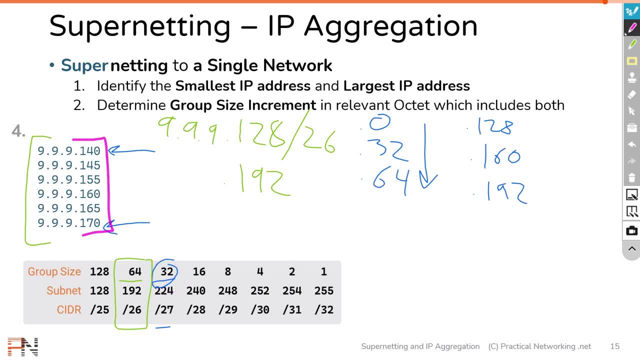 doesn't necessarily mean that's going to be the right size to include all the IP addresses you mean to include. This is similar to the third visualization exercise we did in the beginning of this video, So feel free to check that out if you're unsure. what just happened? 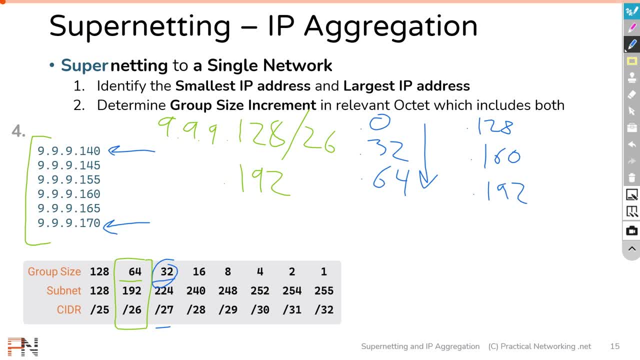 As for us, we're going to continue Now. so far, all of the subnetting problems we've done together have all fallen in the fourth octet. What I'm going to show you next is how to do supernetting problems that involve the third octet. 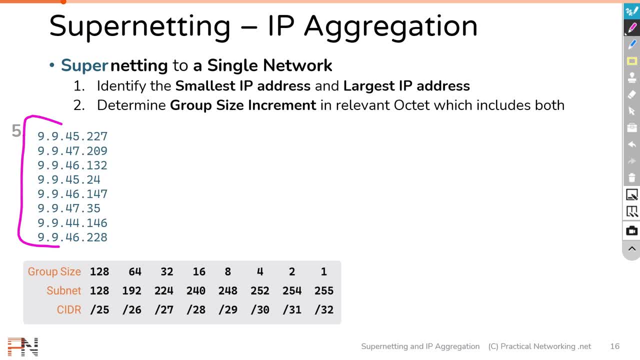 We are now going to summarize these eight IP addresses that involve different third octets. Now, of course, if we're going to the third octet, we need to extend our subnetting chart. one more line, And again I discuss how to do this in video six of the subnetting mastery series. 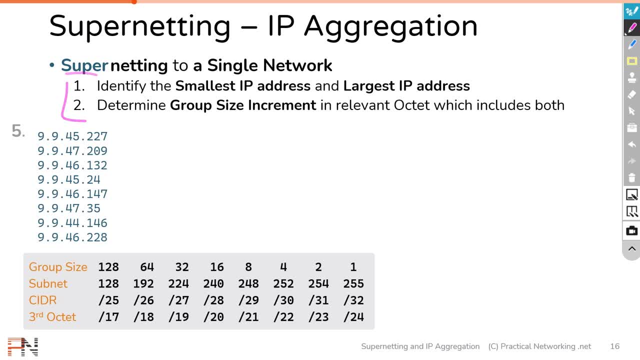 From here we can use the exact same two-step process to supernet these eight IP addresses. Now again, we'll start by finding the smallest IP address and the largest IP address. The smallest IP address for us- looks like this guy- And the largest IP address for us. 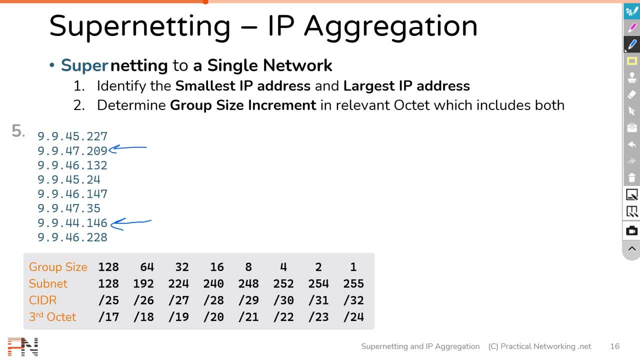 looks like this guy. So if we write that out to make it a little bit easier to see, we have 9.9.44.146 as our smallest IP address and 9.9.47.209 as our largest IP address. 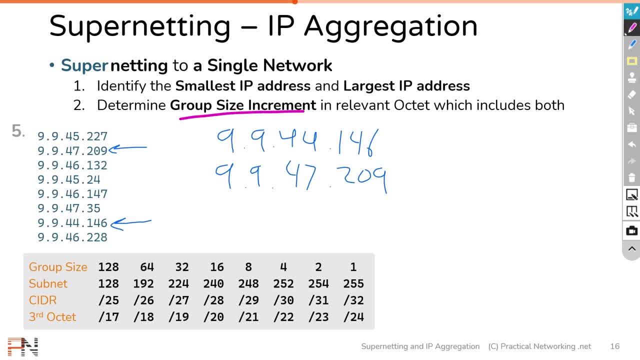 Now we just need to find a group size increment that's going to span these two IP addresses. But notice the steps say in the relevant octet, Since there are different values in the third octet. the third octet is the relevant octet. 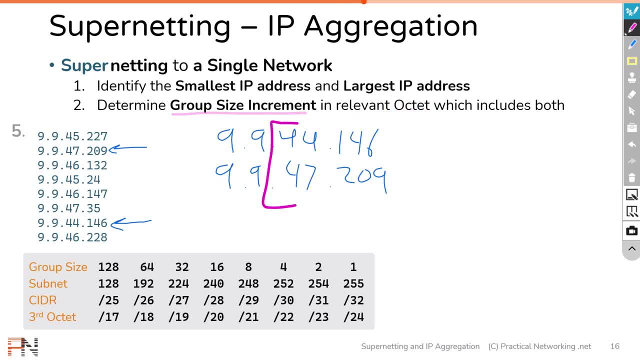 which means I'm trying to find a group size increment that'll span 44 and 47. Now if we subtract out 47 and 44, we get three. That lets me rule out those two sizes right there, which brings me to this column over here and a slash 22.. 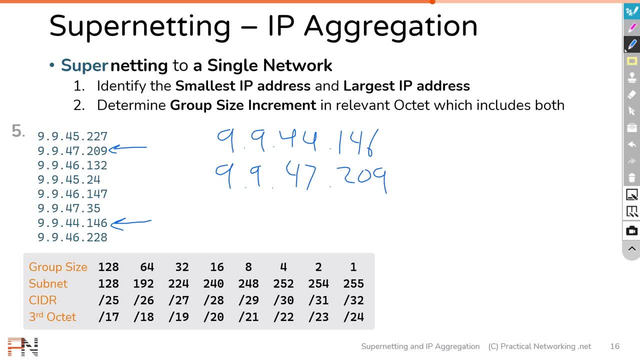 Let's see if a slash 22 will work Again. a slash 22 has an increment of four in the third octet And we can use one of the speed tips that we learned in video five of the subnetting mastery series to start at dot 40.. 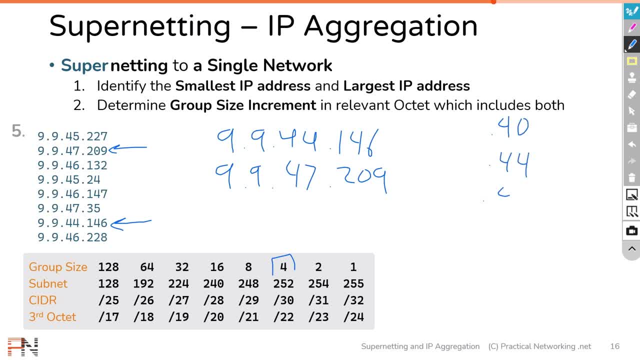 From there we can go to dot 44 and then dot 48. And just like that we have found a jump which includes the IP addresses. we need to summarize, Which means the answer to this supernetting problem is going to be 9.9.44.0 slash 22.. 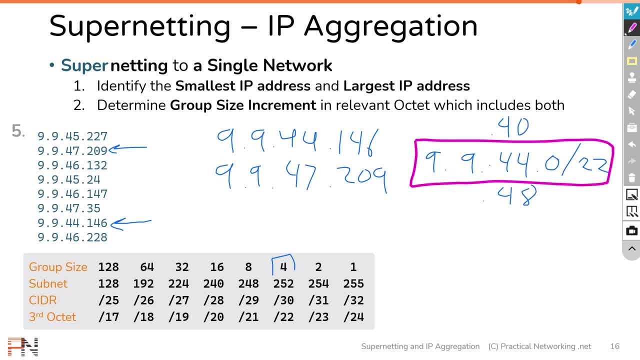 Just like that. we have solved a supernetting problem using these two steps and the third octet. So you see, no matter what these two steps are all you need And, at the end of the day, all you're doing is finding an increment. 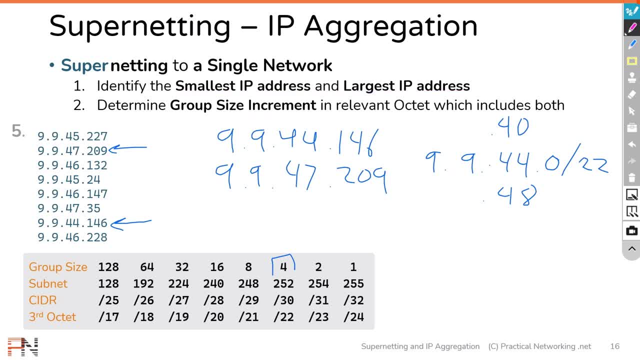 which includes a smallest IP address and the largest IP address. The last problem we're going to work through together involves another problem using the third octet, except this time we'll be solving for mixed networks that span both the fourth and the third octet. 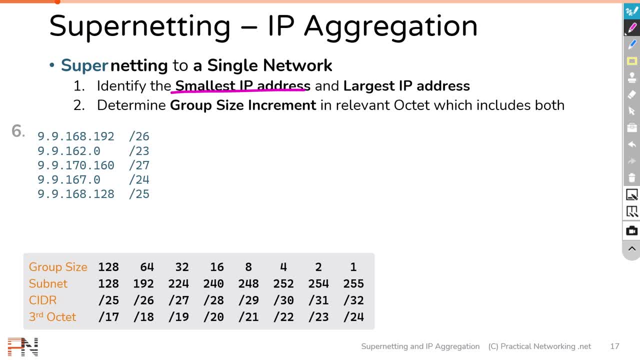 Again. we'll start the exact same way. We'll find the smallest IP address and the largest IP address. Well, the smallest IP address is going to be the network ID of the lowest numerical network, which looks like that guy right there, which means our smallest IP address is going to be: 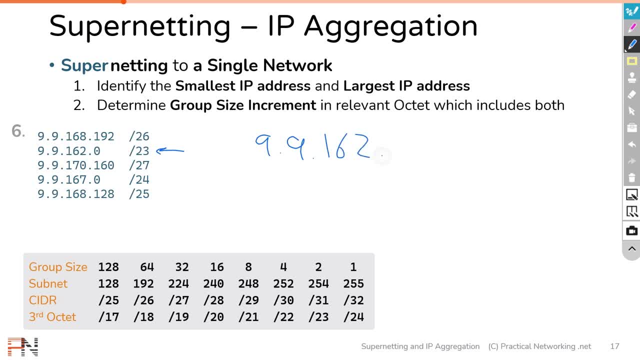 9.9.164.0.. And our largest IP address is going to be the broadcast IP of the highest numerical address, which looks like that guy right there. That is a slash 27 network If we look at our subnetting chart. 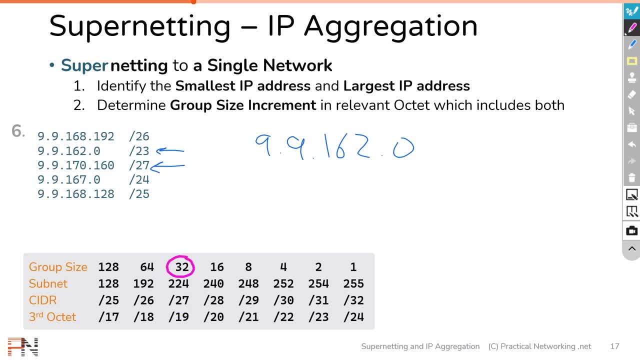 a slash 27 is an increment of 32.. And since this is a slash 27,, we're incrementing that in the fourth octet. So if we add 32 to 160, that gets us 192. And then we do minus 1.. 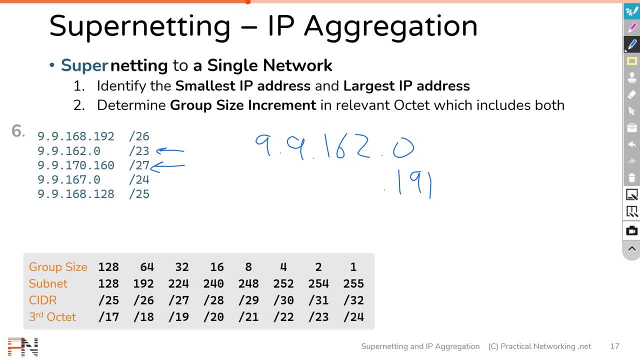 That gives us a broadcast IP address of 191.. And then, if we fill in the remaining octets, we know that the largest IP address in this subnet is going to be 9.9.170.191.. Now we can move on to step 2,. 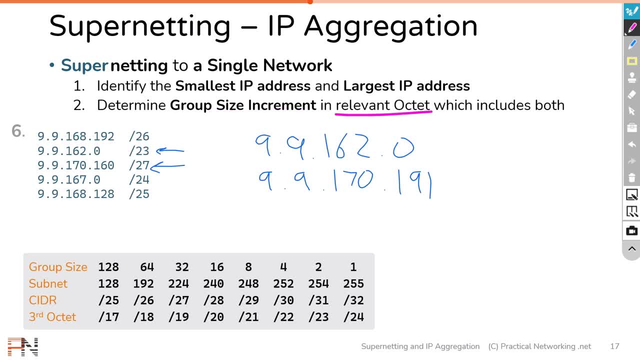 which is to find a group size increment in the relevant octet, which includes both. But you have to be careful with this one. If we subtract 170 from 162,, that would get us 8,, which would bring us to a slash 21.. 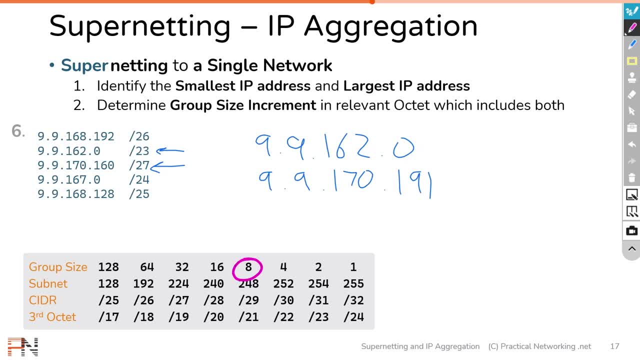 But you have to be careful here, because 8 would be a jump from 999.162.0 through 999.170.0.. It wouldn't include .191.. We actually need to find a jump that includes 8 in the third octet. 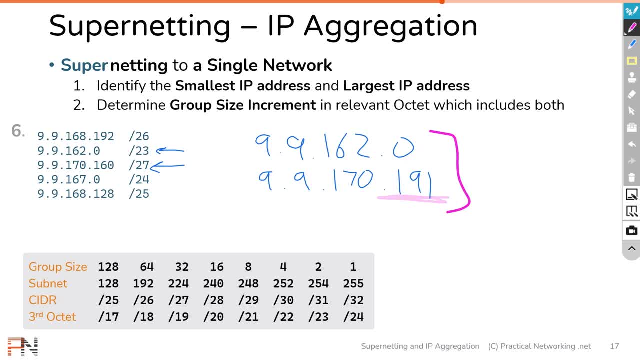 plus a little bit more to account for our fourth octet. So 8 is actually not going to be big enough for this particular supernetting problem. So we have to go a step further, all the way to slash 20, which gives us an increment of 16.. 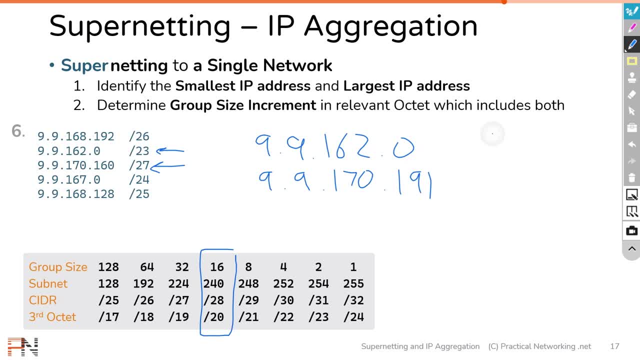 And again, we can use a speed tip of multiplying it by 10 to let us start at 160. And if we increase that by 16, that would mean that the next network would be 176.. But right, there, we have found a jump. 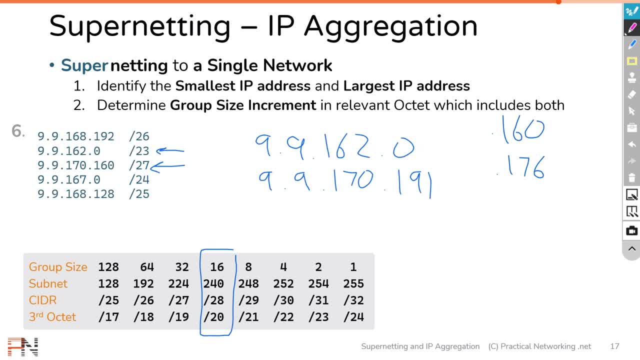 that includes both the smallest and largest IP address. And so right there we have our answer of 9.9.160.0 slash 20.. Just like that, we were able to solve using only scratch paper and our handy subnetting chart. 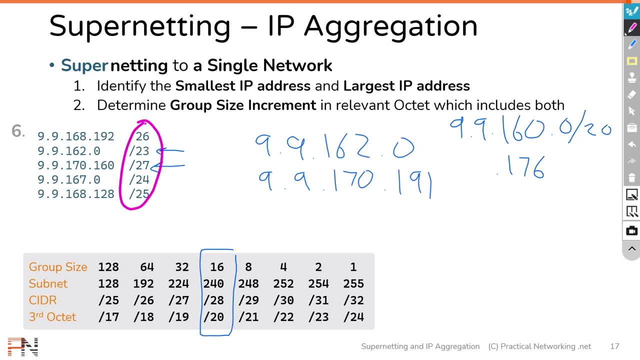 another supernetting problem that involved mixed-size networks in the third and fourth octet. At this point we've worked through six supernetting problems together, using only pen and paper and our handy subnetting chart. Hopefully by now you feel pretty good. 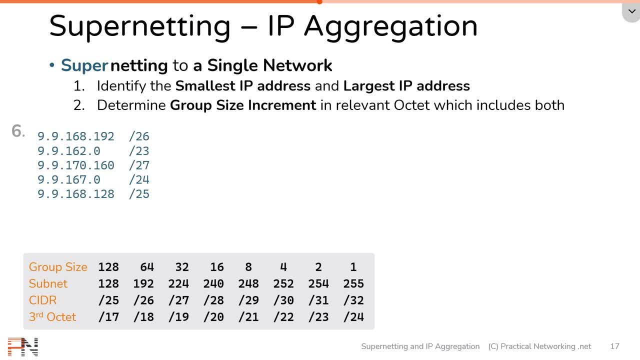 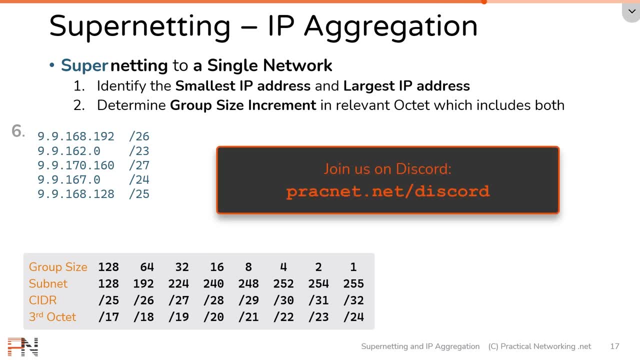 about how to solve supernetting and aggregation problems. As I said before, mastery doesn't come without practice, So find a buddy and give each other summarization problems so you can practice together. A great place to find such a buddy is our new Discord server. 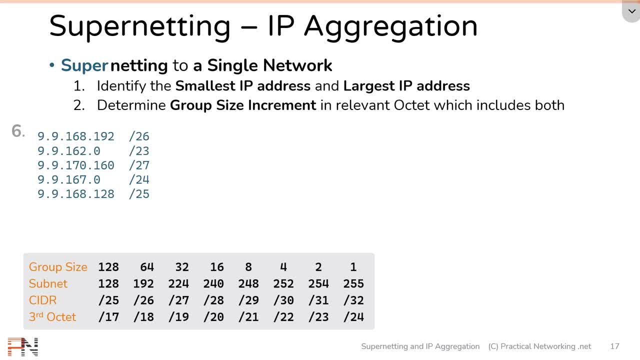 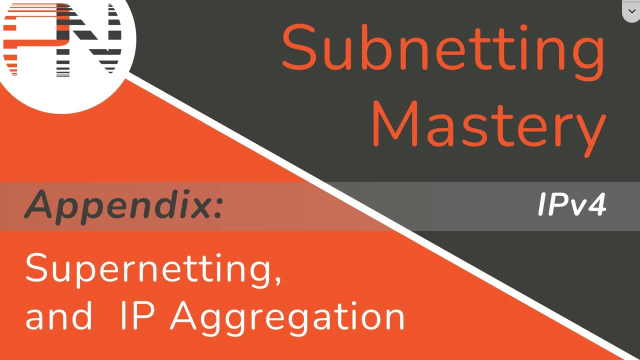 Join us at pragnetnet. slash Discord. And that, my friends, brings this lesson to a close. I hope you enjoyed this lesson on supernetting. Please don't forget to show your support by giving this video a like, subscribing and mentioning in the comments. 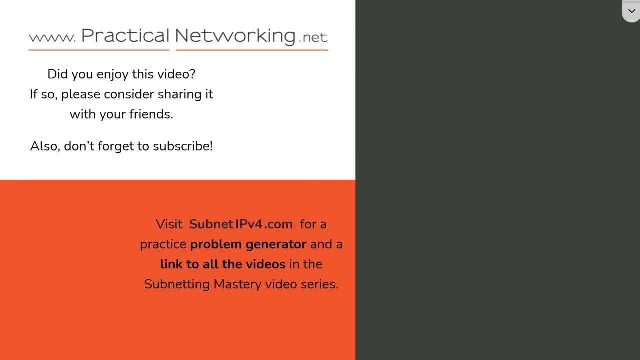 something you want to learn. next, Of course, the best way to show your appreciation is to share this video with a friend. If you're studying for the CCNA, check out pragnetnet slash CCNA for a bunch of free, high-quality resources.